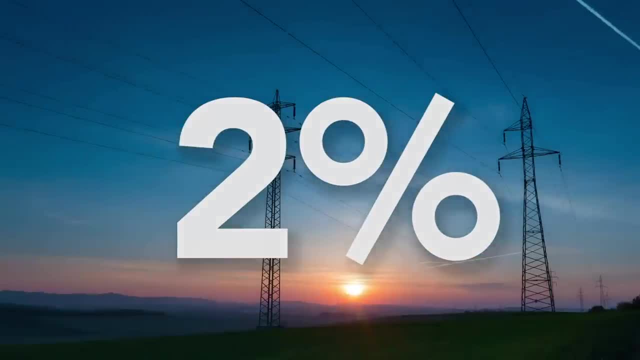 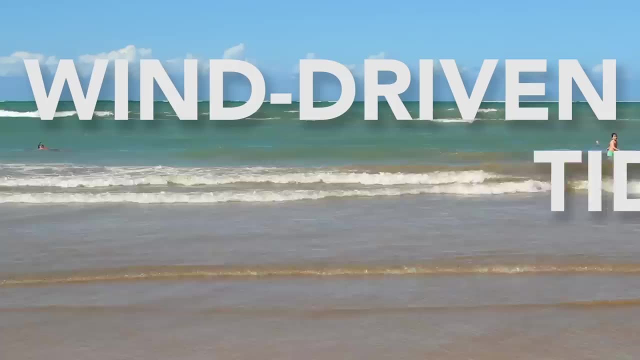 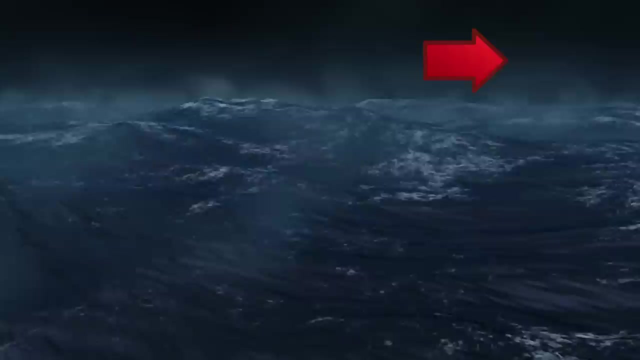 In fact, just two percent of the total energy of ocean waves could be used to power the entire world. There are essentially three types of waves: Wind-driven waves, tidal waves and tsunamis. Wind-driven waves form as wind passes over the surface of the water. Pretty simple Energy from 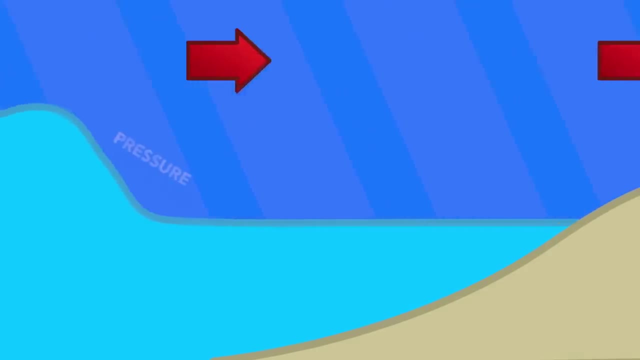 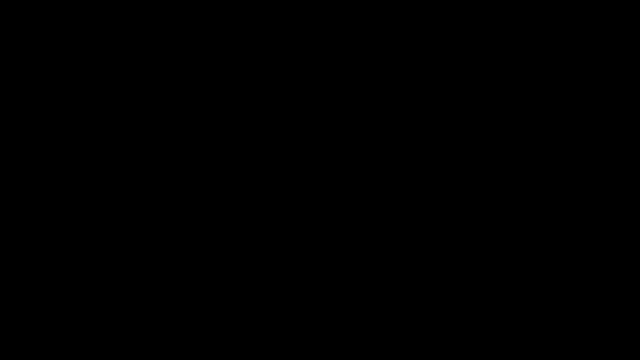 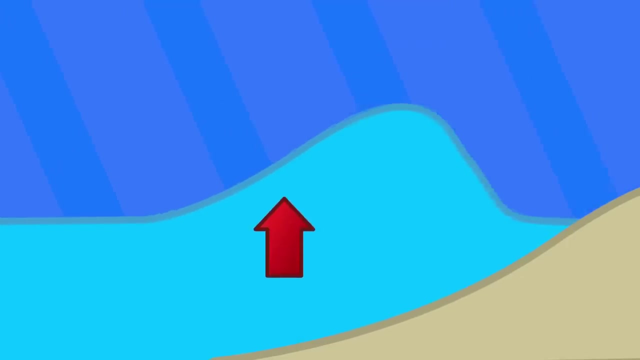 It's the wave that moves through the water. In general, This means that as a wave moves through the water, the water itself essentially moves up and down, reacting to the wave energy moving through it. So wind can cause waves through friction and pressure. But there's also another. 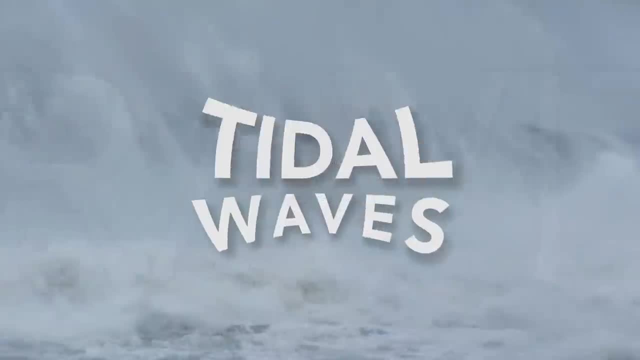 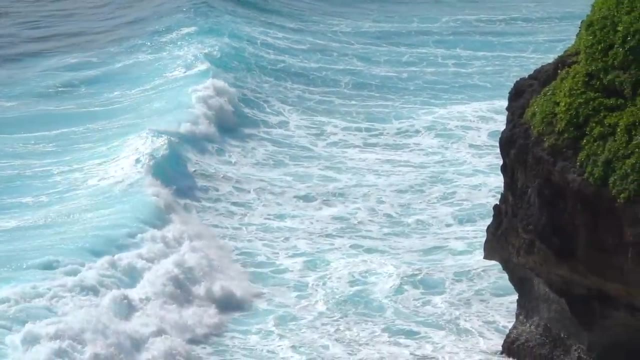 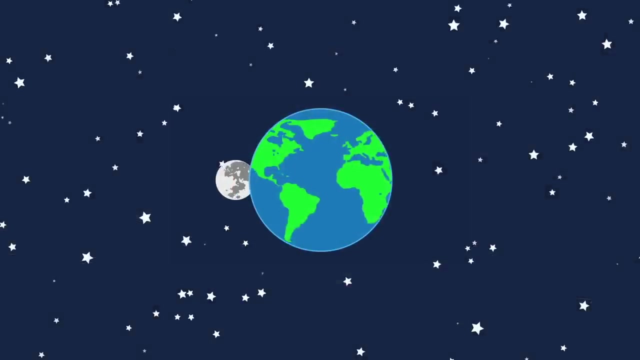 hidden force to certain waves. Gravity Tidal waves are not massive tsunami-like waves like you may be thinking. These are actually just large waves that move across our planet. The gravitational forces of the earth, sun and moon- affect how the water on the earth behaves. The moon has the greatest effect on waves. 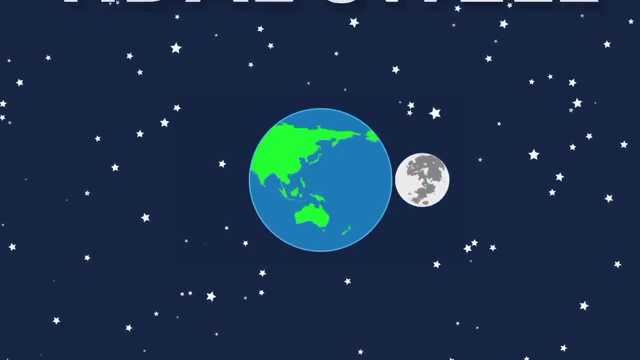 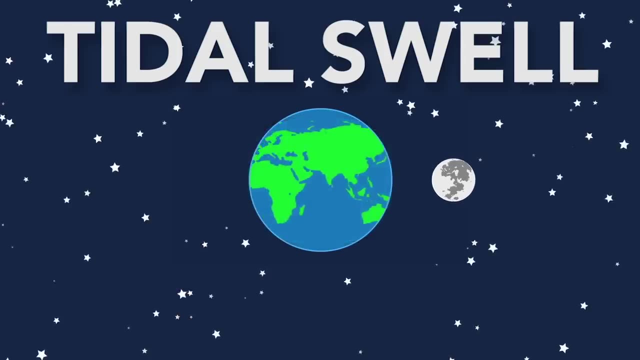 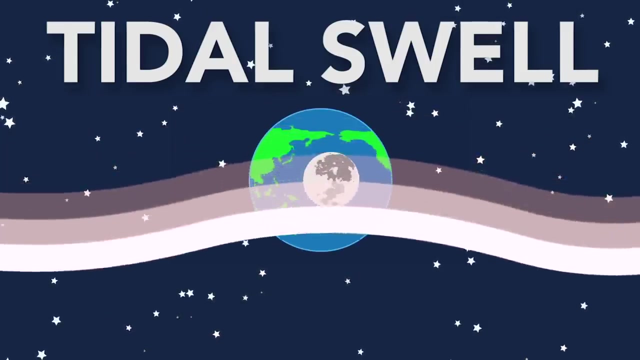 as it moves around the earth. As the moon moves, it causes oceans to swell on either side of the earth or the side closest to the moon and furthest from the moon. As the earth rotates, tides around the world go in and out, as we all probably know The actual mechanics of this. 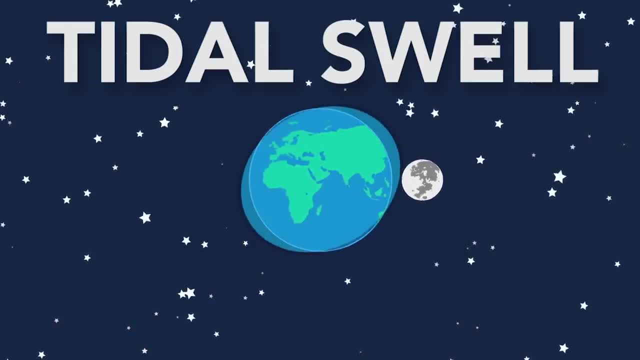 might surprise you, though, The bulge of the water on the earth stays consistent with the location of the moon, and it's actually the movement of the earth that greatly affects tides going in and out. This gives the appearance of high and low tides, when in actuality, it's the earth that's. 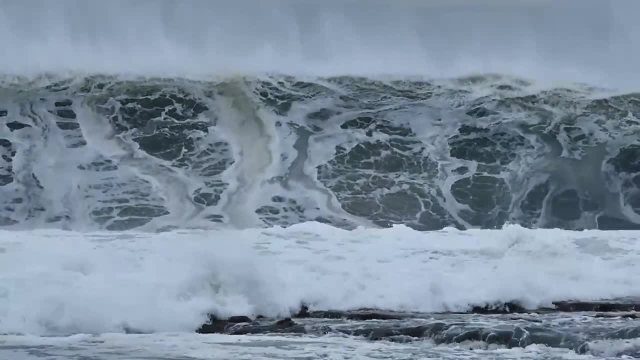 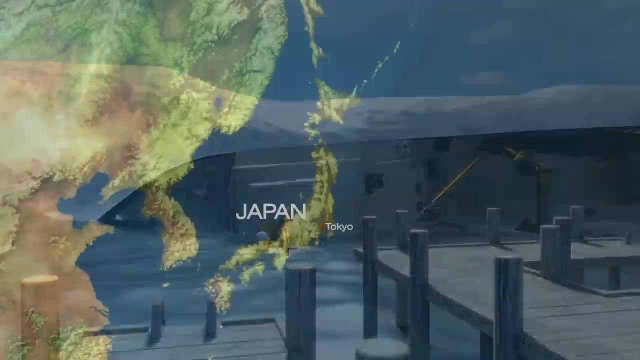 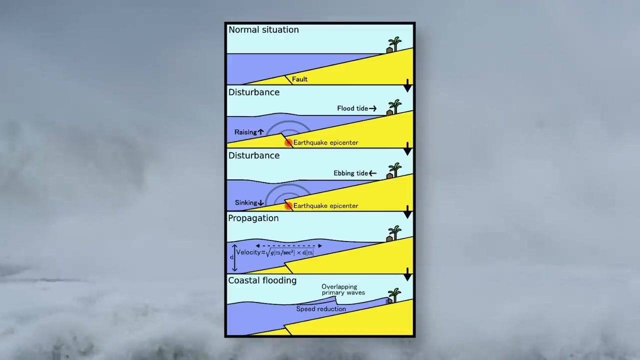 moving, not the water. The last type of waves to discuss are abnormal in nature. Tsunami waves are large, powerful waves caused by geological disturbances like earthquakes, landslides or volcanic eruptions. Tsunamis are generally very large simply due to their nature and